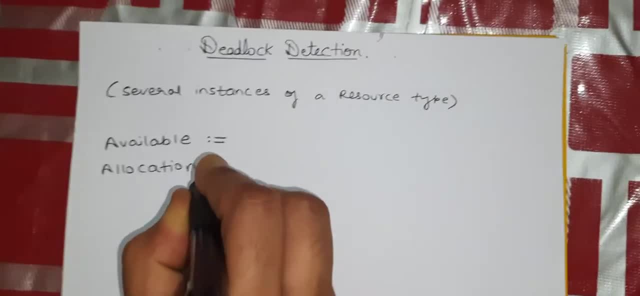 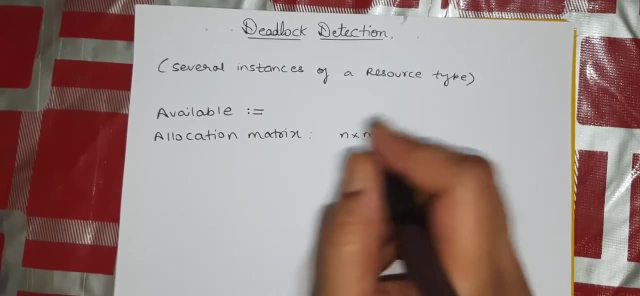 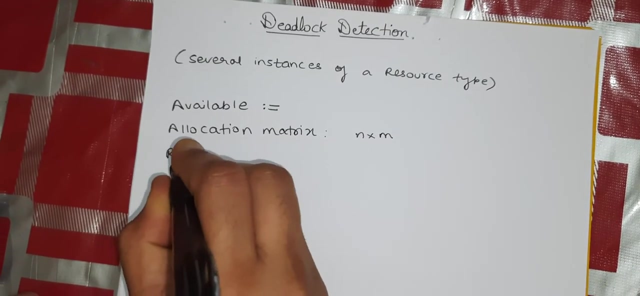 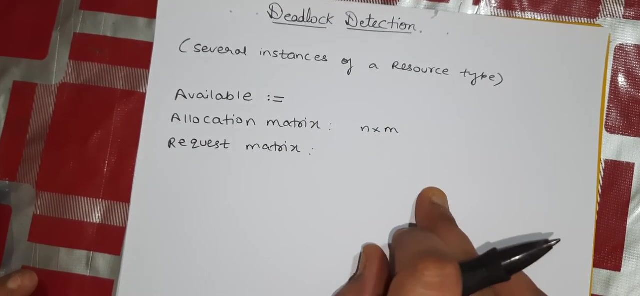 Next we are having the allocation matrix, right? So again, allocation matrix is a n cross m matrix which defines the number of resources available. So it is a number of resources of each type currently allocated to each process, right Again. next, we are having one request matrix. So here we are having the request matrix. It is also a n cross m matrix which indicates the current request of each process. 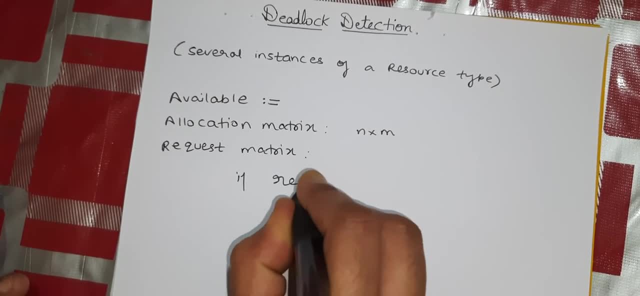 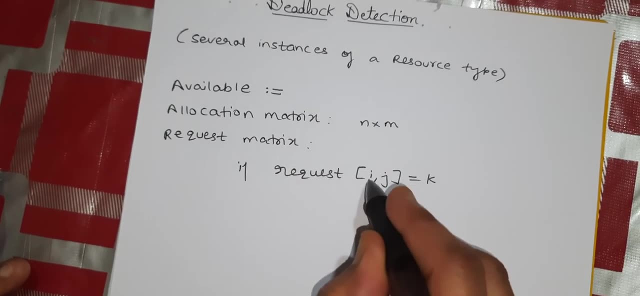 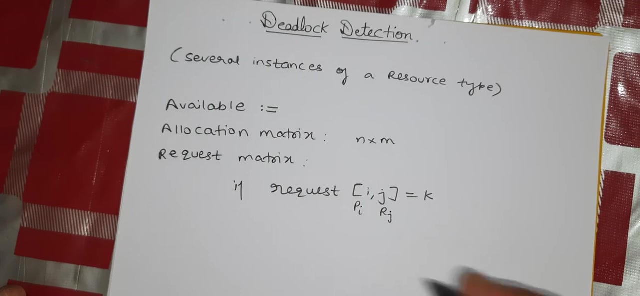 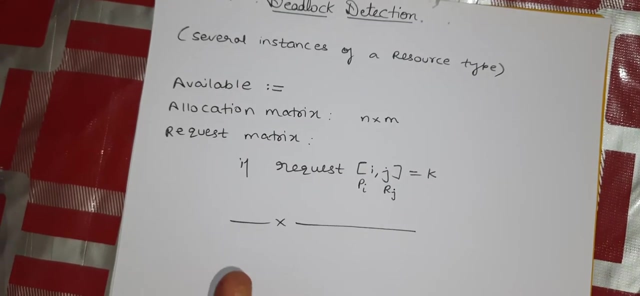 That means if request i, comma j, equals to k, then it means that process. So request pi is requesting k instances of resource type Rj. right Now, apart from this, these data structures or these variables, we use in the algorithm, let's see the algorithm, the deadlock detection algorithm. 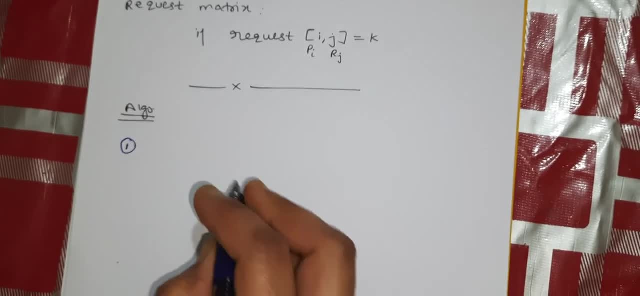 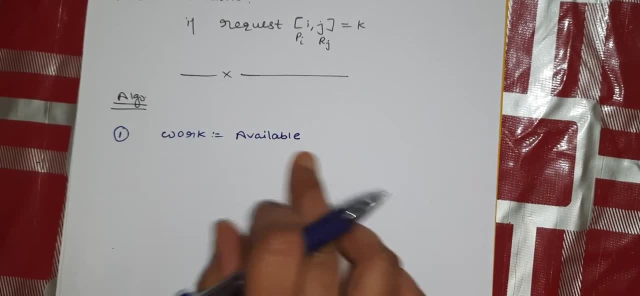 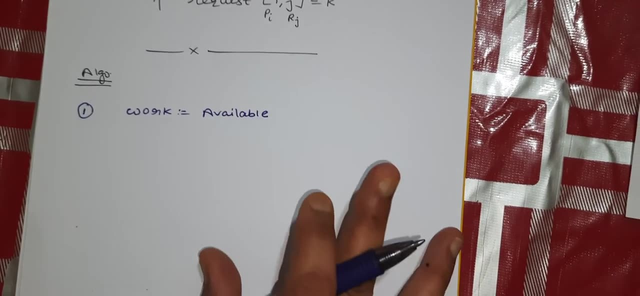 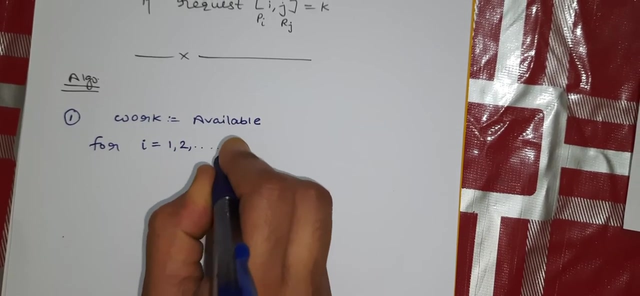 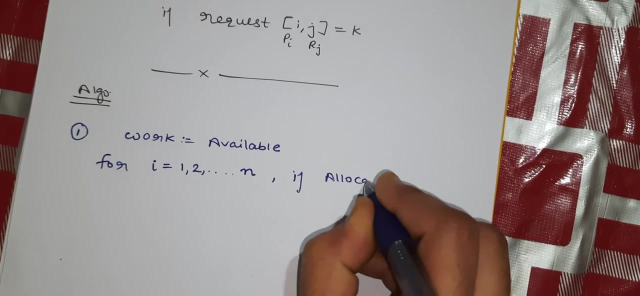 We work with FD, the algorithm, with the number of resource type available, the number of instances of each resource type we are having. we are available right. so for each process, processes, and we are having n processes and it is denoted by i, so for each process we'll see that if allocation of ith 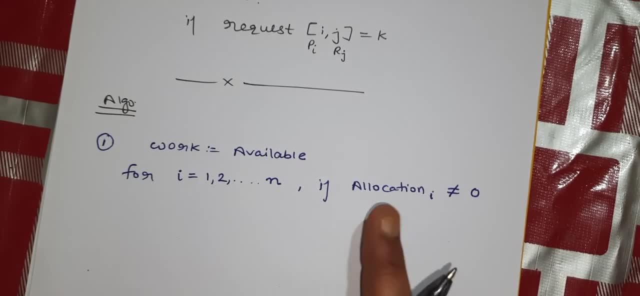 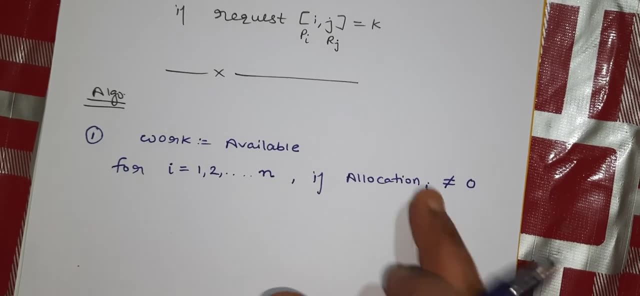 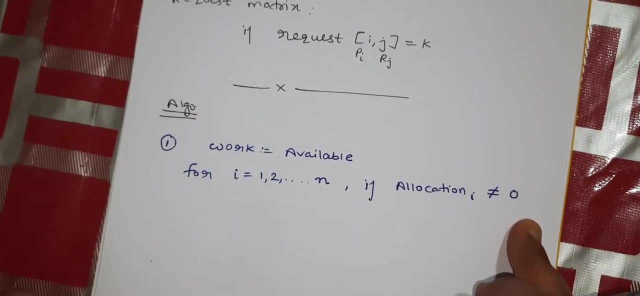 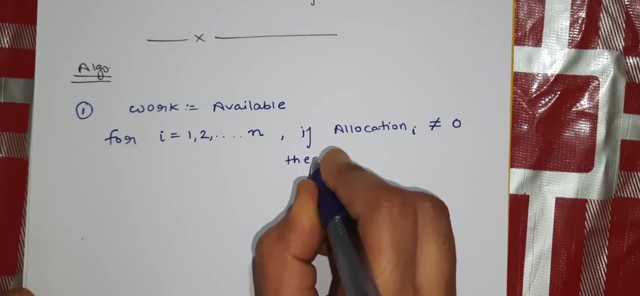 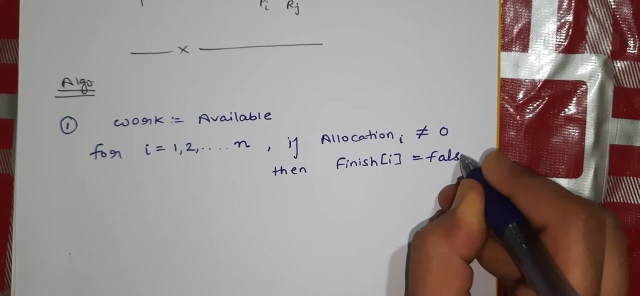 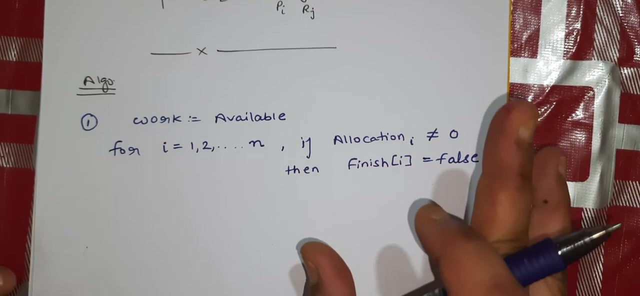 process is not equals to 0. what does it mean? it means that if we are, we had allocated some resource, some instances of resource type, to ith process. right, that means allocation is not equals to 0. Because if it is completely executed, then its finish is true and it has not allocated any resource. 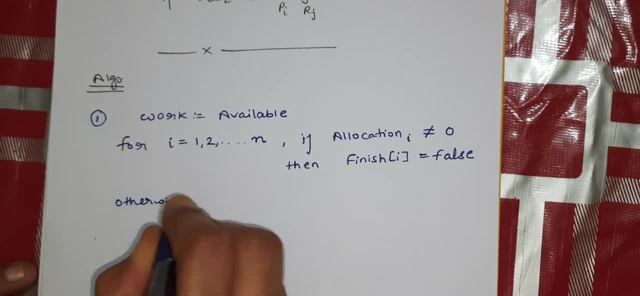 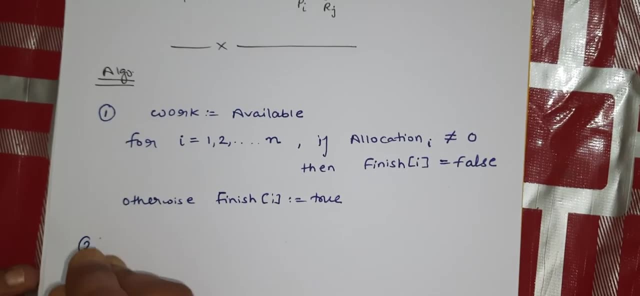 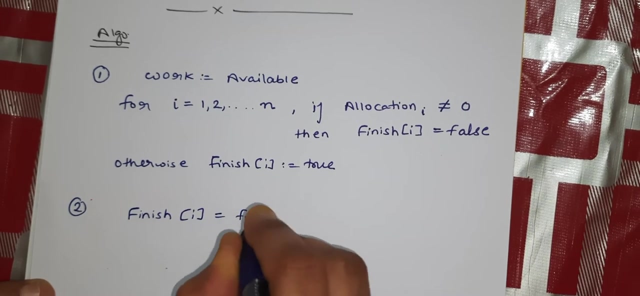 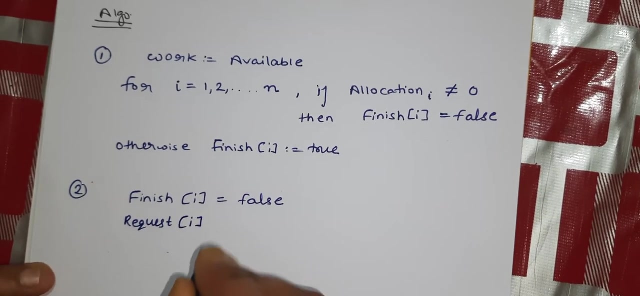 Otherwise the finish of the ith process would have been true. If the finish is false, then you check three things. First, the finish of the ith process is false. Then you check what is the request of that ith process, Because we have a request matrix here. Every process is requesting for some additional resources. 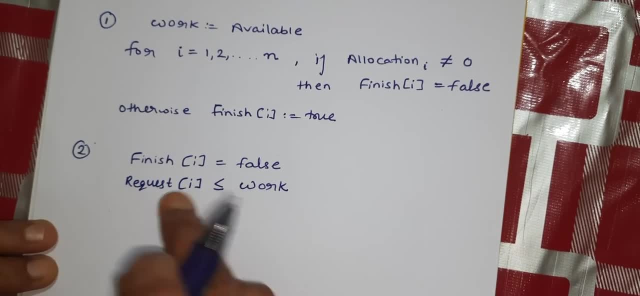 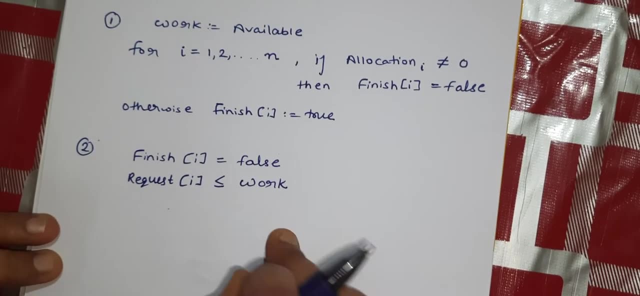 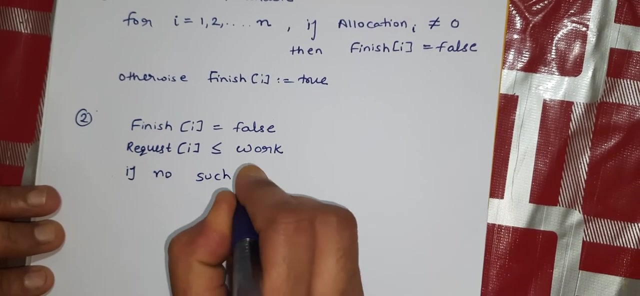 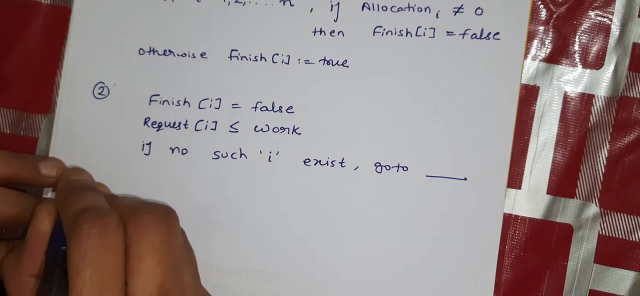 So the request of the ith process check if it is less than or equal to work. Are the instances of resource type available sufficiently? If it is, then you go to step 3.. Then you go to step 4.. And if there is no such request of any process, then you go to the last step. 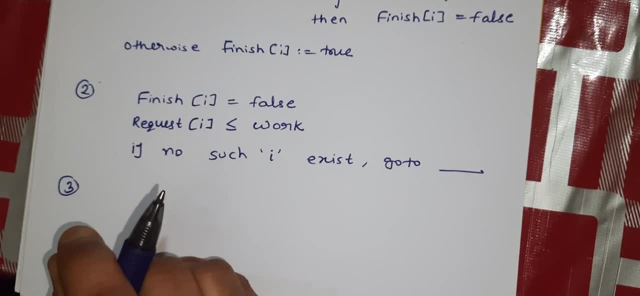 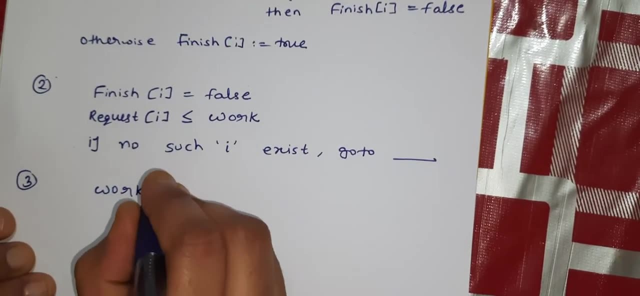 Otherwise you go to the next step. So if you are able to satisfy the request of any process, then what will you do? When you satisfy its request, then that process will be completely executed. And when that process is completely executed, then what will it do? 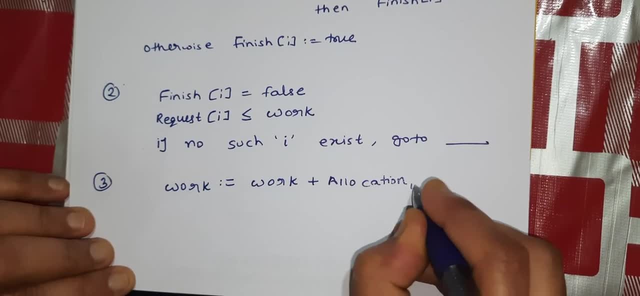 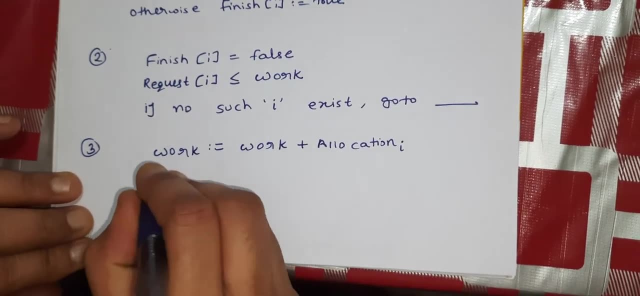 The resources it had allocated. it will release the resources And when it releases the resources, where will they go back and be added? They will be added to the work And after being added, what will you do? You will true the finish of that process. 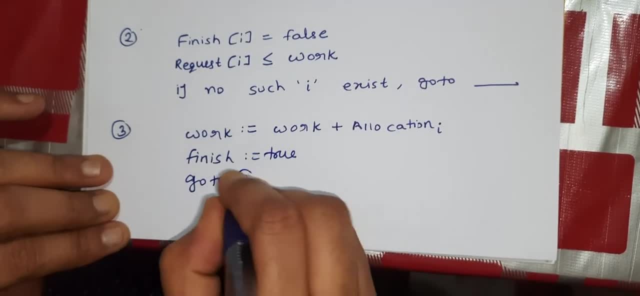 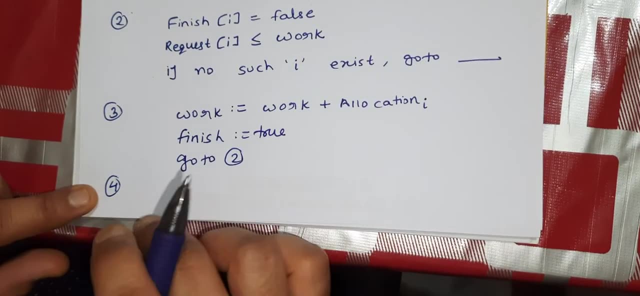 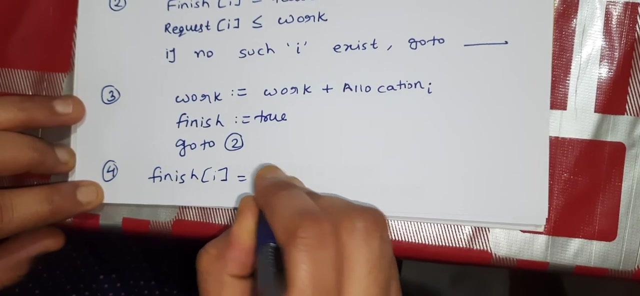 After true, what will you do? Where will you go back? You will go to the previous step. You will check for the next process again. And what else will you do? If you have false the finish of that process, then you will check in the last step. 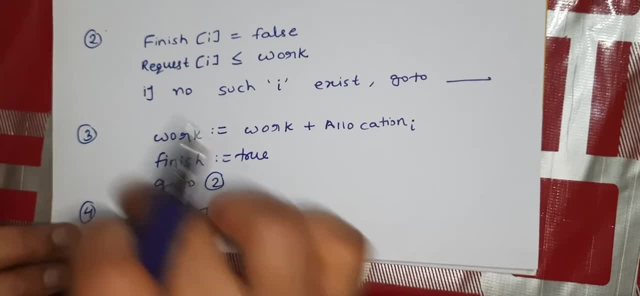 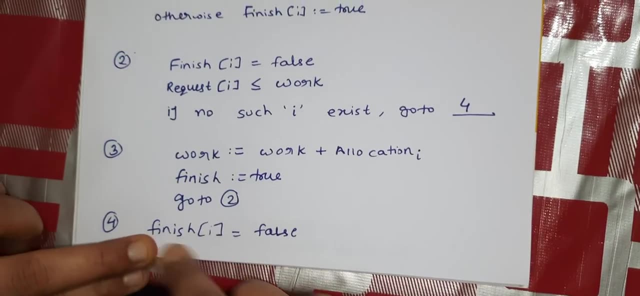 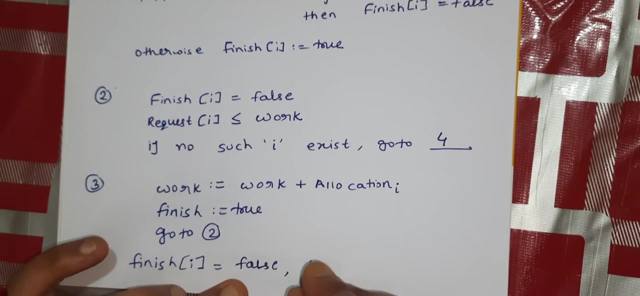 Is there any process whose finish is false. So if, even after repeating it, if you have checked at last, even after repeating it, is there any process which has not been completely executed, So if the finish of any process is false, it means that your next process is deadlocked. 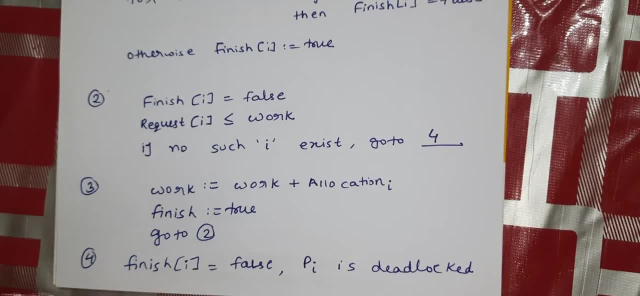 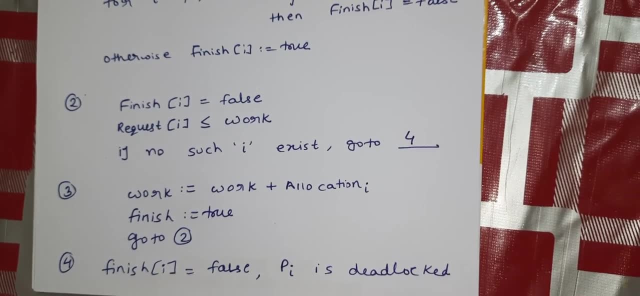 It is in the deadlocked state, So you can detect the deadlock Right. Because if the finish of all the processes is true, it means that no process is in the deadlocked state, But if any process is left, it means that you are not able to satisfy the request of that process. 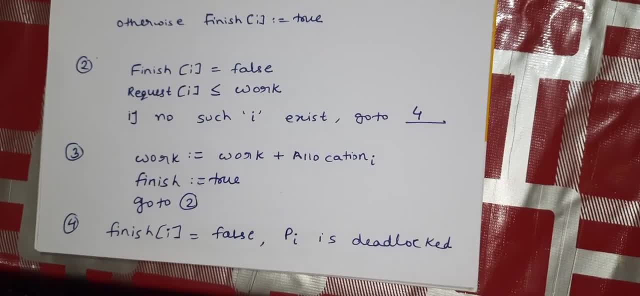 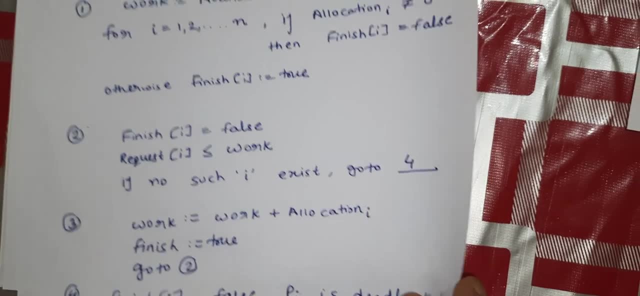 And that process is in deadlocked state, Right. So let's see one example on this Deadlock detection. through this, Multiple instances available, Right. So again, we will see the same scenario As we are having in the banker's algorithm. 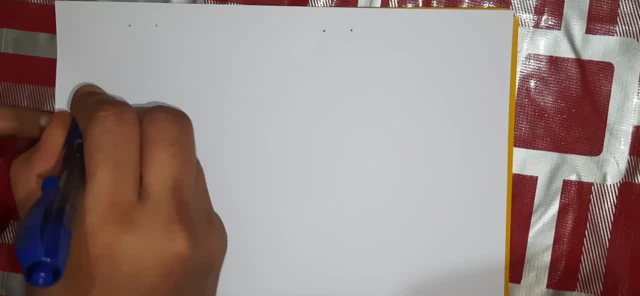 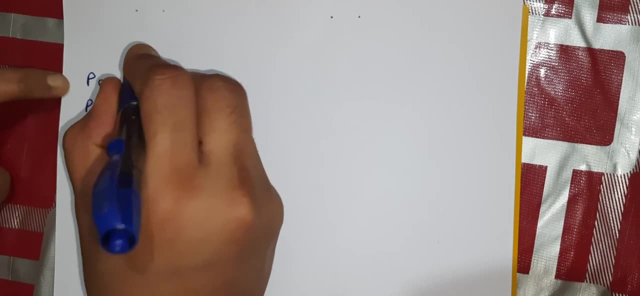 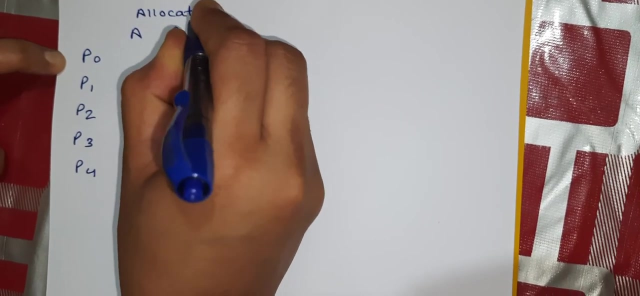 we are having the resources: P0, P1, P2, P3, P4.. We are having the resource types. We are having three resource types: A, B, C, Right, And we are having the allocation matrix. 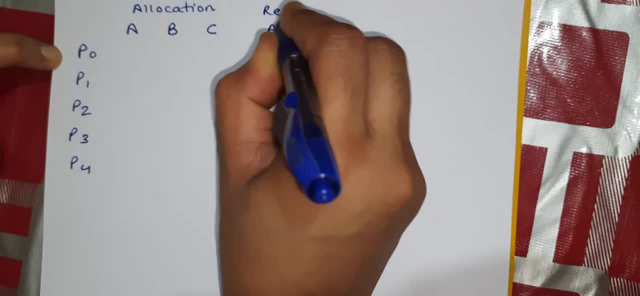 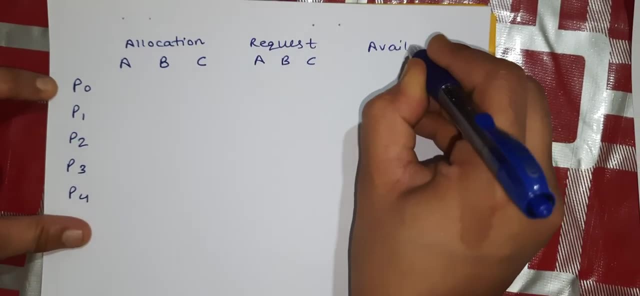 Similarly, we are having the request matrix Right, So we are having these two matrices available And we are having the available. So either we are given with the total or we are given with the available. So if we are given with the total, 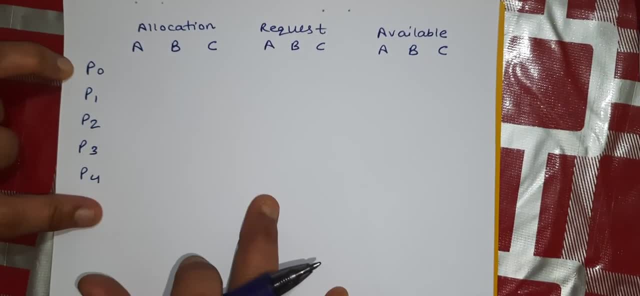 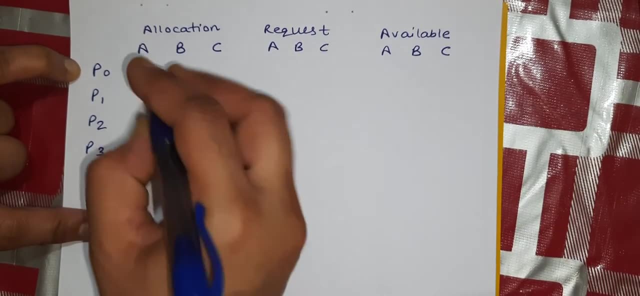 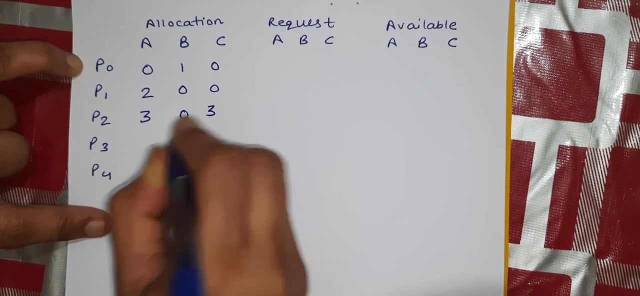 what we will do. We just sum up these allocation and we subtract from total minus allocation. We get the available and sometimes directly we are given with this available. So this is 010, 200, 303, 211, 002.. 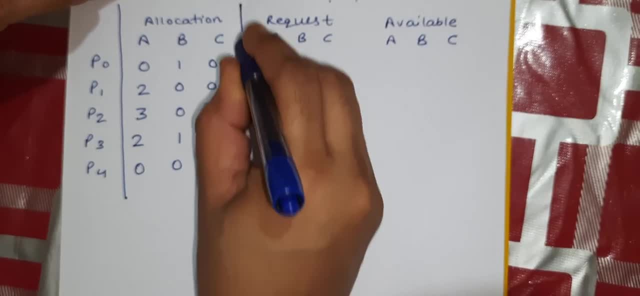 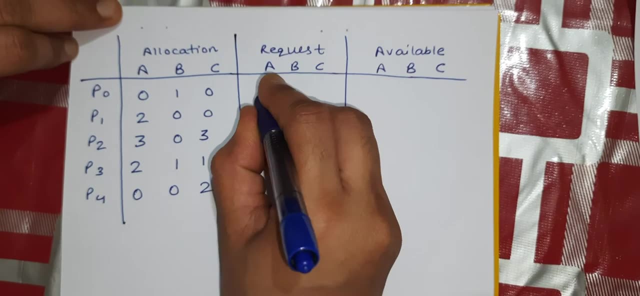 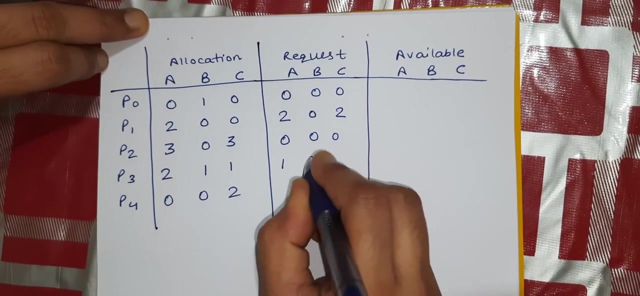 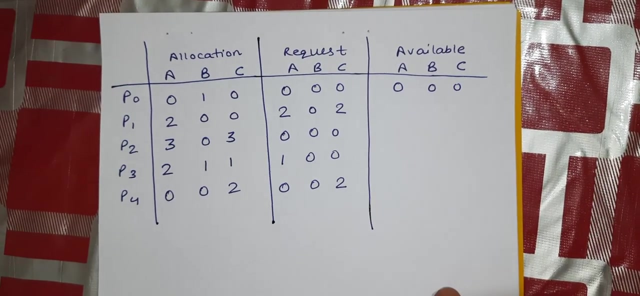 This is the allocation matrix Right Now. request matrix is 000, 202, again 000, 100, 002.. Right And available is nothing. All the resource types instances available. We had allocated all the resource types. 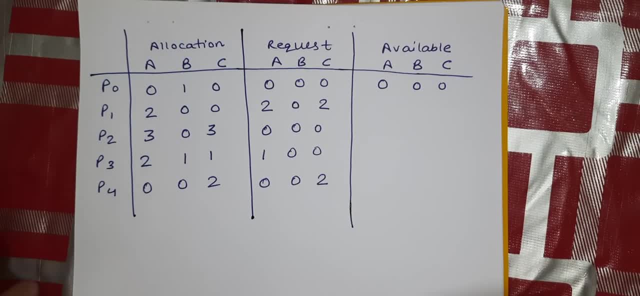 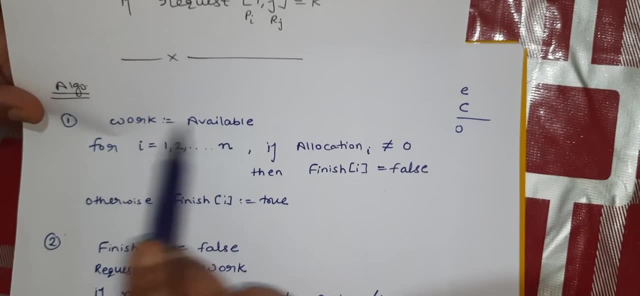 So now we have to check that, whether the system is in deadlock state or not. So how we will see With this algorithm, initially work is equal to available. So what we will do, We check that if allocation is not equal to 0,. 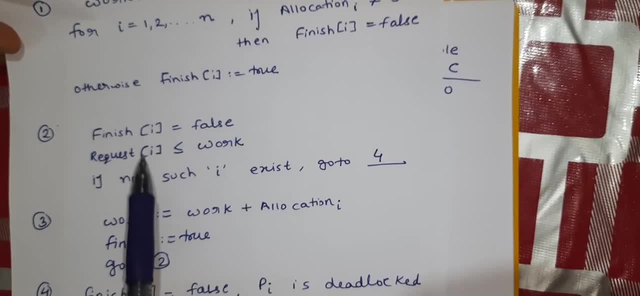 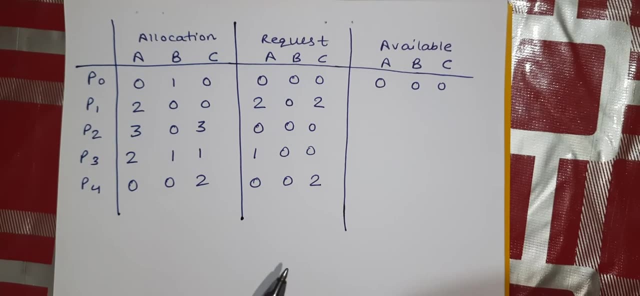 that means that process is not finished. So, one by one, we pick the process and check that whether we are able to satisfy its request or not, Right. So initially, when we see that P0 process is requesting for nothing, when it is requesting for nothing, 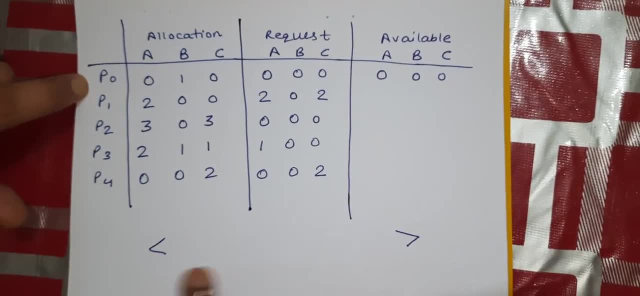 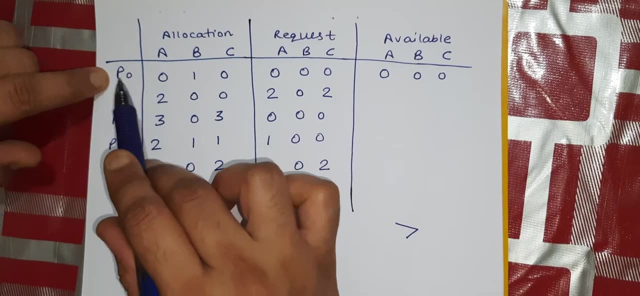 and initially no processes had been finished. this sequence is empty, Right? So when? because it is requesting for nothing and nothing is available also. So what we will do: This process will get completely executed, And when it gets completely executed, 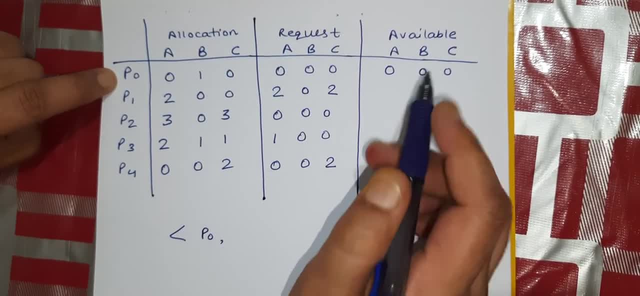 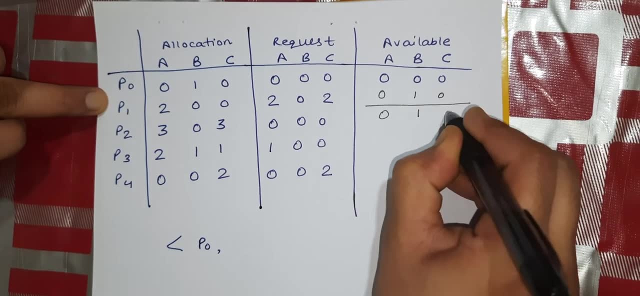 we just add its allocation into the available. So what we will do? We just add this 010 into this available. So now available is 01 and 0.. Right, So P0 process is completed. Now we will go to the P2 process. 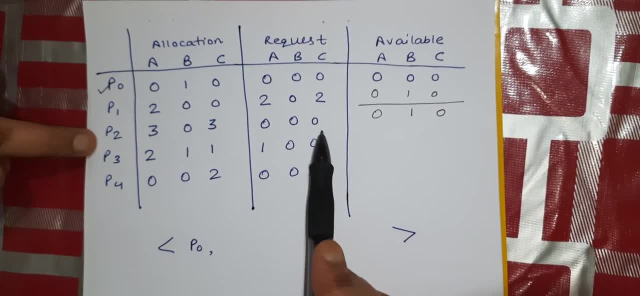 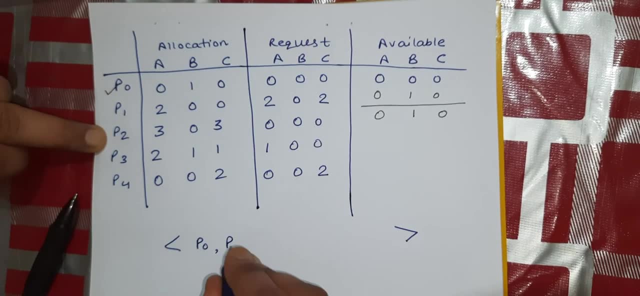 So it is not less than available. Now again: P2 process request. P2 process request. for nothing That means we can also able to execute the P2 process. So we execute the P2 process and its allocation had been allocated to the. 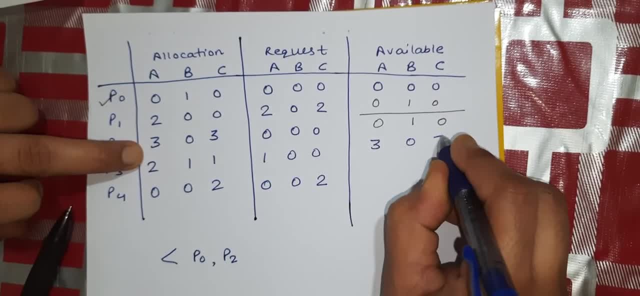 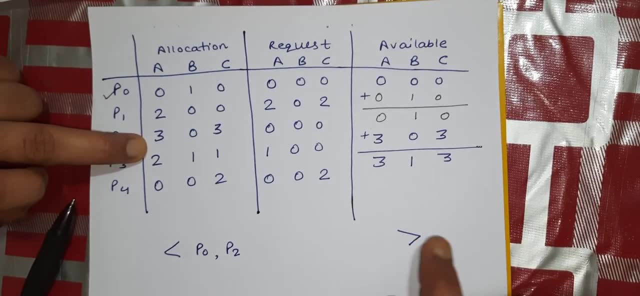 added to the available, So its allocation is 303.. So we just add up this, So now we are having 313.. Now it is available. Now afterwards, when these are available, we check the request of P3 process. It is. 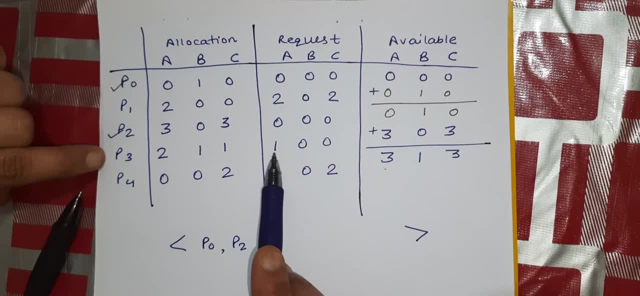 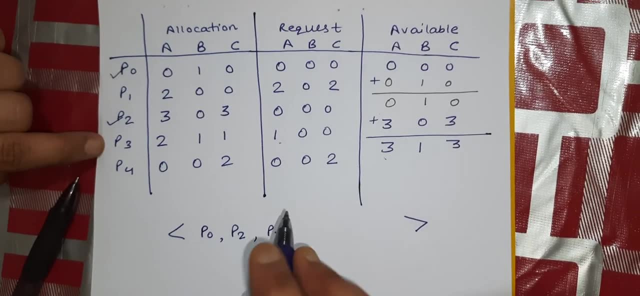 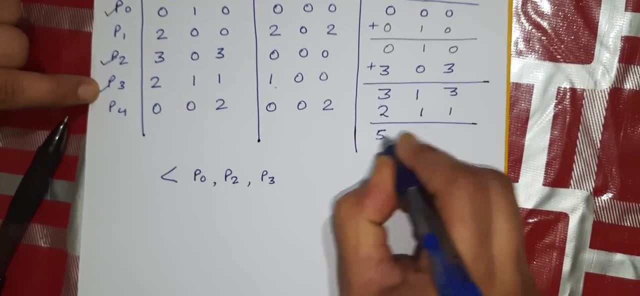 it can also be satisfied Right, Because it requests only one instance of resource type A. So that means next we can satisfy the P3 process. So when P3 is executed we can add this allocation to here, So we are having 524.. 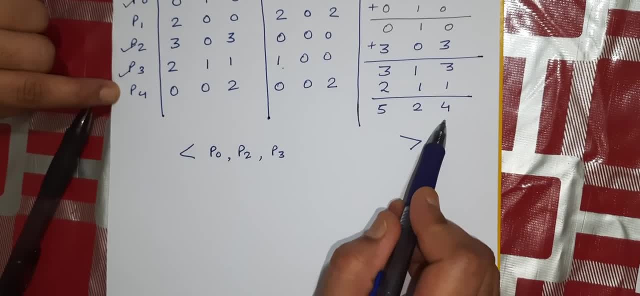 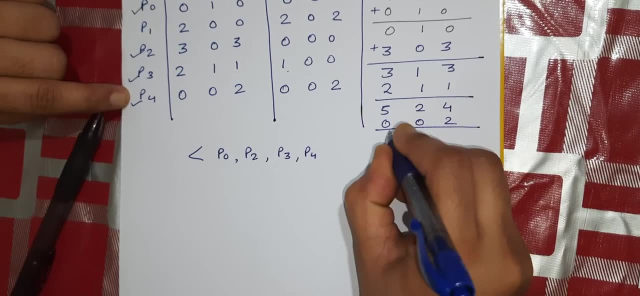 Now again it requests for two instances of C resource type. It is available So we can complete. for P4 process Again. its allocation had been added here, So we are having 524.. Finally, when we go back to P1,, 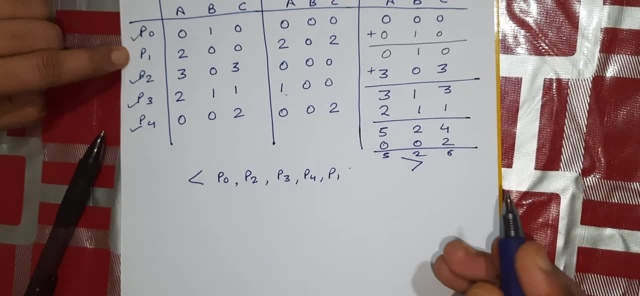 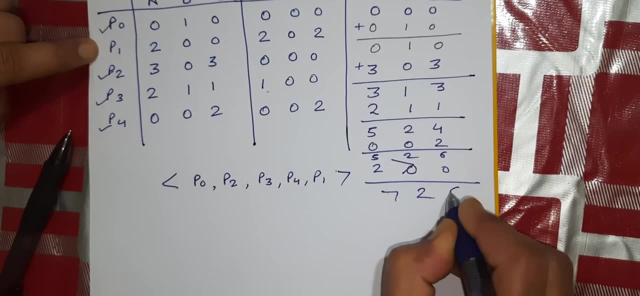 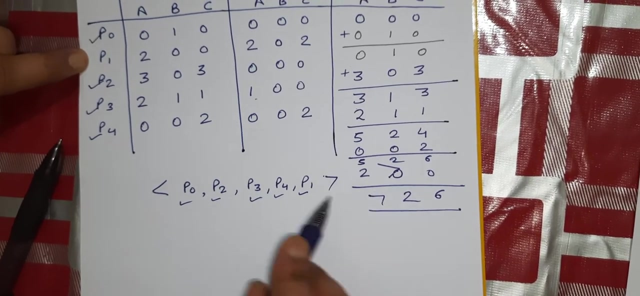 now again sufficiently available So we can have P1 process here and the allocation of P1 had been added to here. So we are having 7,, 2 and 6.. Now all the processes are in this. All the finish of all the processes, is true now? 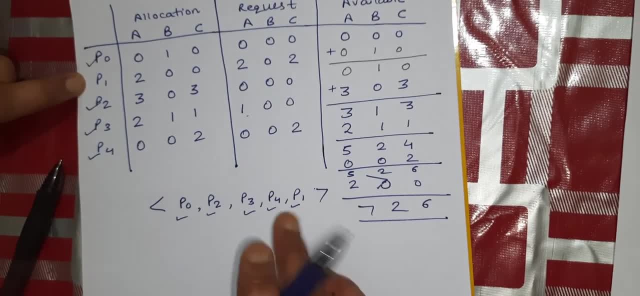 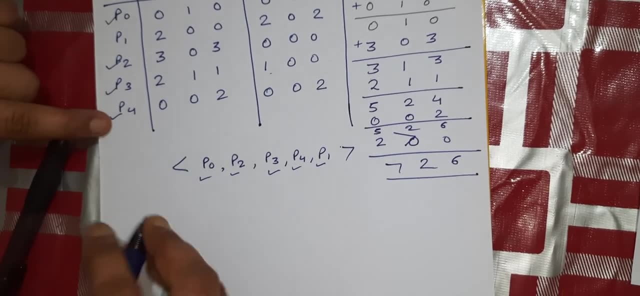 0,, 1,, 2,, 3, 4.. All the processes finish is true. That means there is no deadlock is detect in the system Right Now. suppose at any instance of time the P2 process made request. 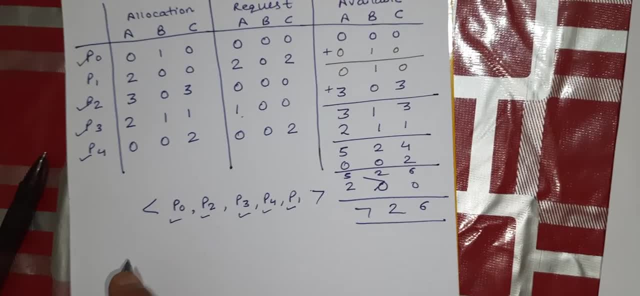 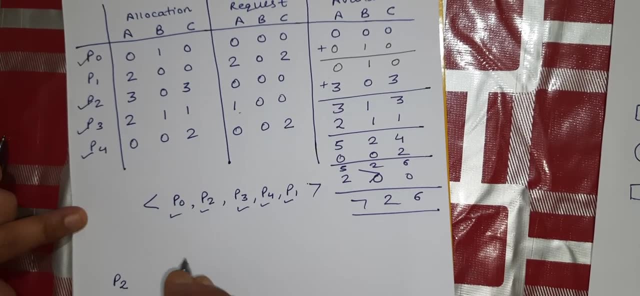 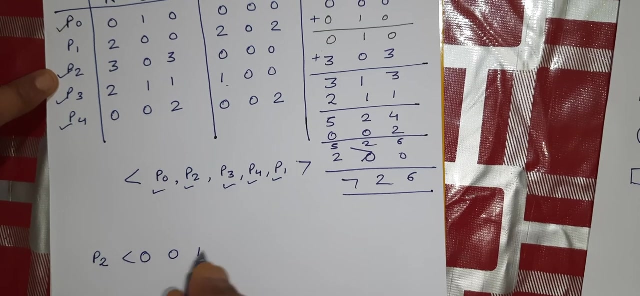 Right. So P2 process made one additional request of like instance of request C Right. So that means here P2 process request for 0,, 0, 1 for C resource type Right. The request is like that. Then what will happen? 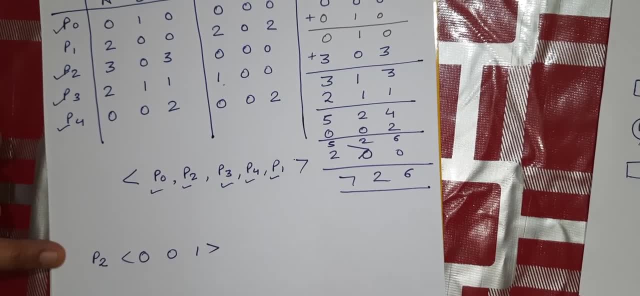 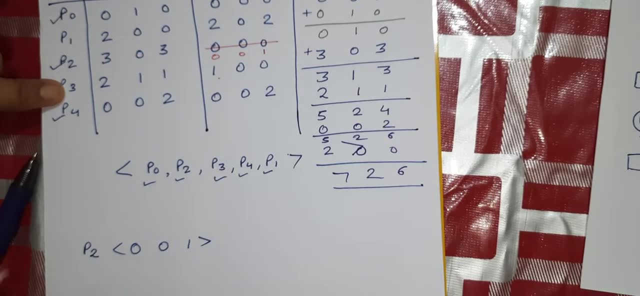 Whether, again, the system is in deadlock state or not. So if it requests for 0, 0, 1.. Now the request is 0, 0, 1.. So what will happen If it requests for 0, 0, 1.. 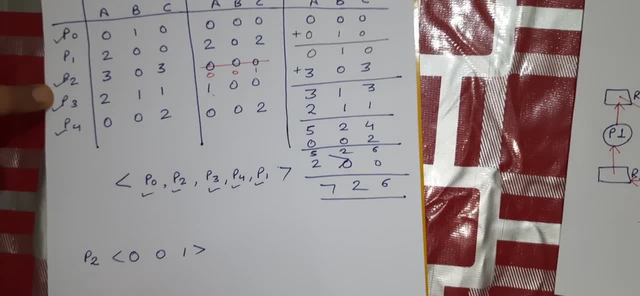 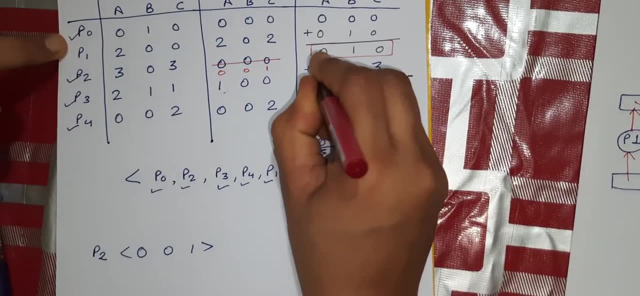 So initially we will be able to execute for P0 process because it requests for nothing, But afterwards, when the resources are released, we are having 0, 1, 0. Right And we are having one instance of B resource type available. 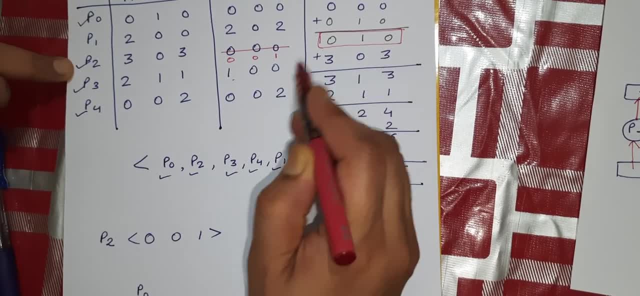 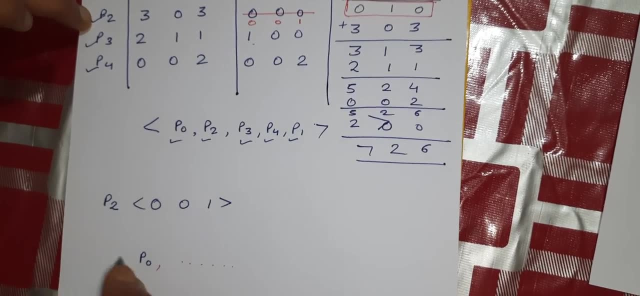 But it is requesting for one instance of C resource type, So afterwards we are not able to execute for any other process. That means in the sequence we are having only P0 process. The finish of P0 process is true only So. that means 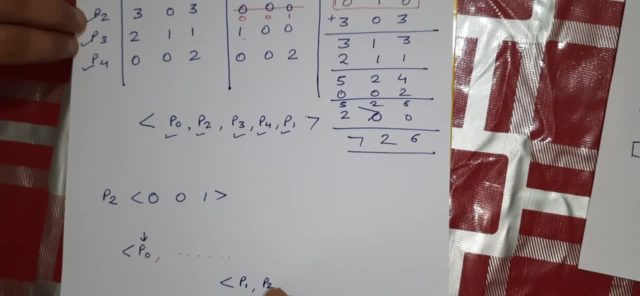 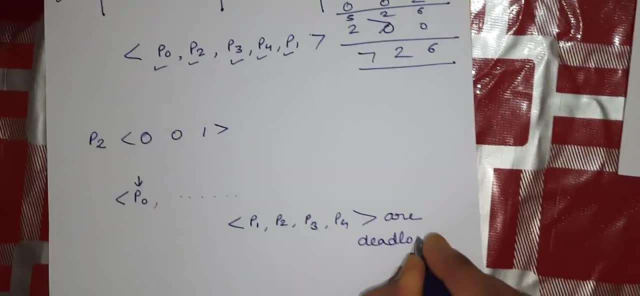 here we can say that P1,, P2, P3 and P4 processes are deadlocked Right. So this way we can be able to detect the deadlock for multiple instances of resource type.